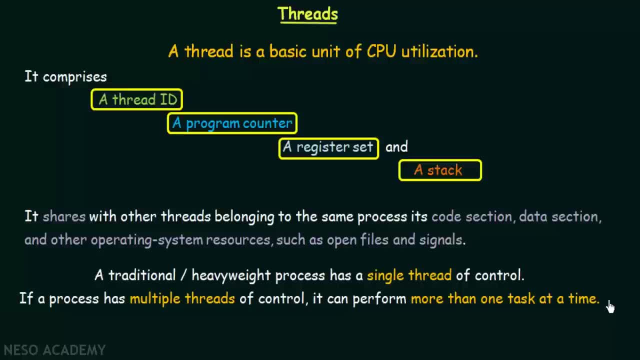 And hence that process can perform more than one task at a time because it is having multiple threads and multiple threads will be performing multiple actions. So there we see how threads becomes useful and how using threads makes the system much more efficient. So here let us try to understand the concept of threads. 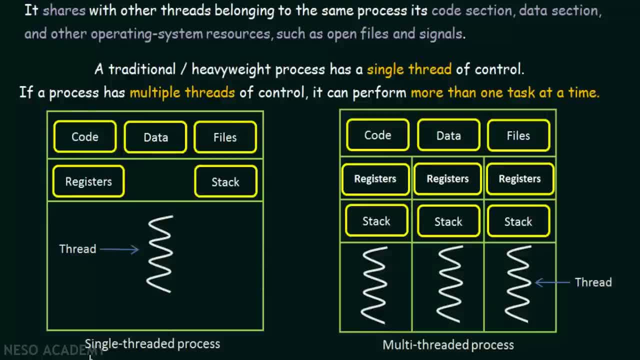 Using these two diagrams. So here in the first diagram it is a single threaded process which we refer to as a traditional or a heavyweight process over here. So here we are having only a single thread, So this whole block is considered as a process. 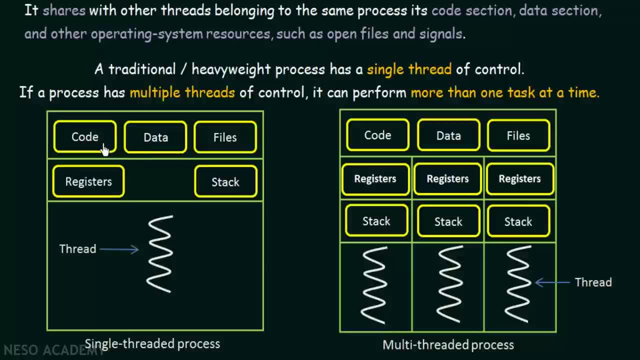 and this process contains only one thread, And this is the code section, the data section, the files, the registers and the stack belonging to this process. So there is only one thread. That means this process can perform more than one task at a time. 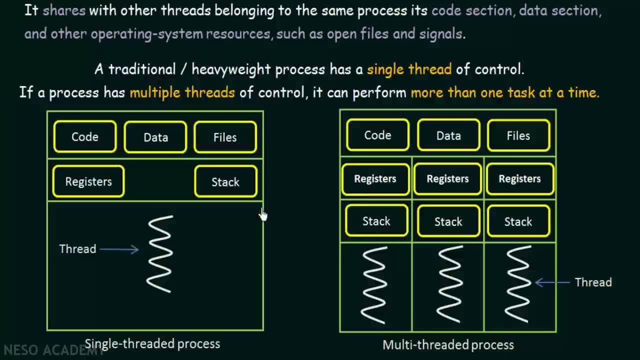 So there is only one thread. That means this process can perform more than one task at a time. So there is only one thread. That means this process can perform more than one task at a time. But in contrast to this, here we have another diagram showing a multi-threaded process. 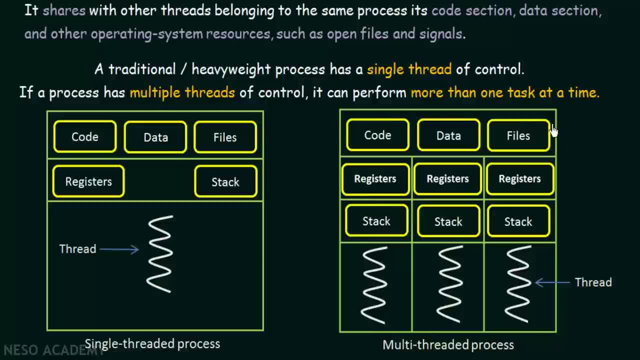 So here this whole block represents a multi-threaded process, So it is a single process and it is having multiple threads over here. So if you see, there are three threads in this process And each of these threads they have their own stack and registers. 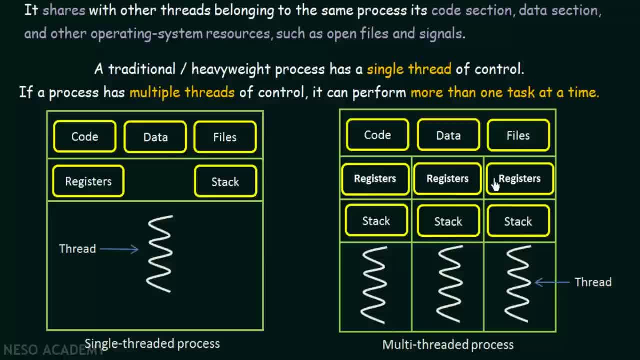 So all these three threads, they have their own stack and registers. So all these three threads, they have their own stack and registers. If you see on top the code section, the data section and the files belonging to this process are shared by these three threads. 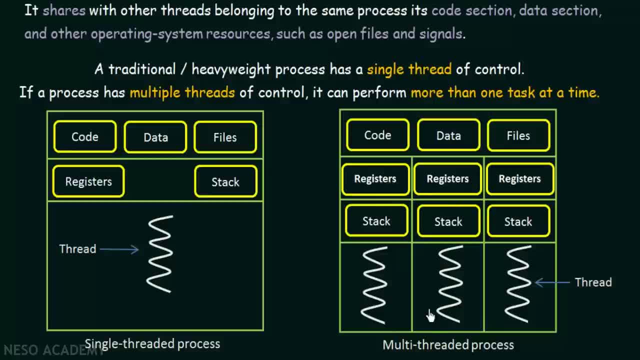 And each thread. they have their own stacks and registers. So this is a diagram of a multi-threaded process. So in this case, this process can perform multiple tasks at a time, Because each thread will performing a different task And hence multiple tasks can be performed at a time. 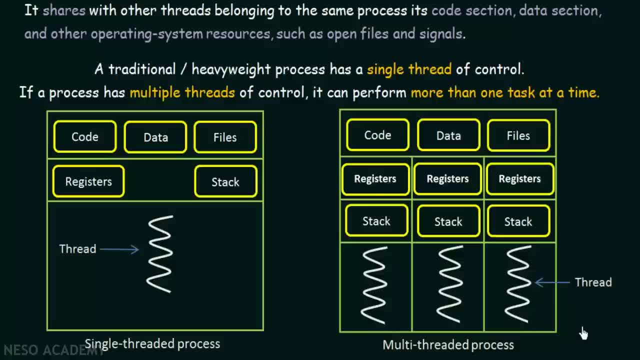 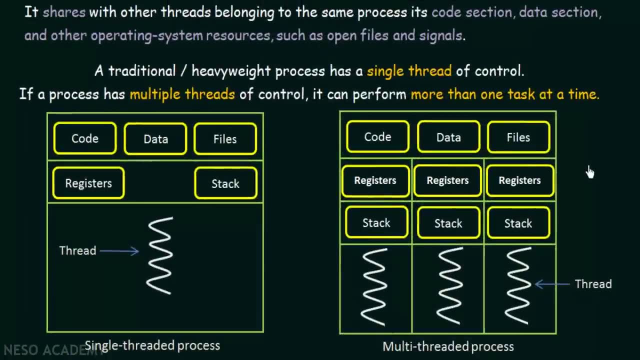 by the help of this multiple load, multi-threaded process. So from that itself we must have understood that it is much more efficient as compared to the single threaded process and it will make our computation faster and more efficient. So in most of the systems that we use today, we follow the system of multi-threaded. 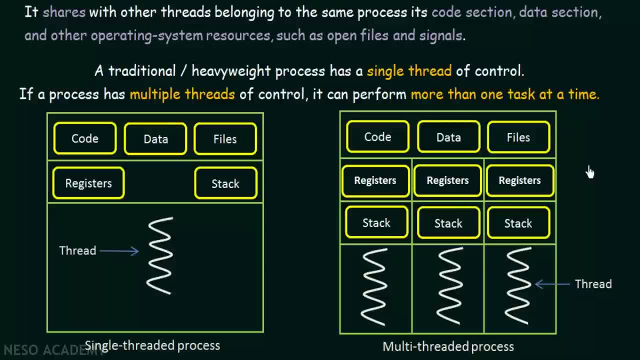 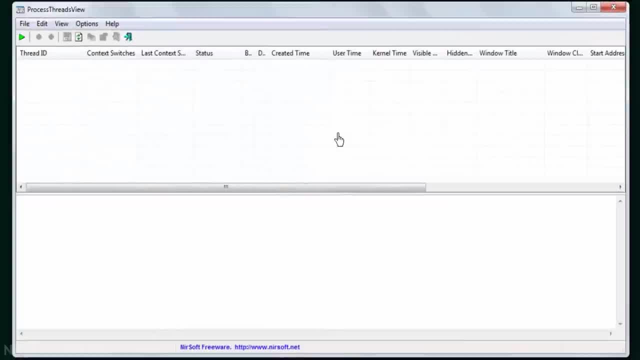 processes. It will be good if we can visually see how it works in our system in order to understand how processes are there and how threads are associated with the processes. So here I have a small software called process threads view, which helps us to see the processes and the 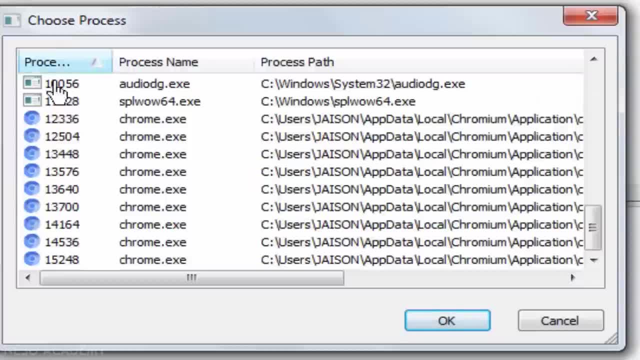 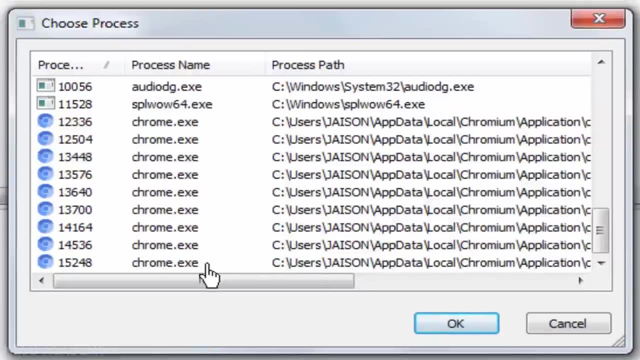 threads running in our system. So if I click here I can see the processes running in my system. So I have opened the Chromium browser in my system, So here I can see the chromeexe processes which are running in my system. So there are quite a few number of chromeexe processes running in. 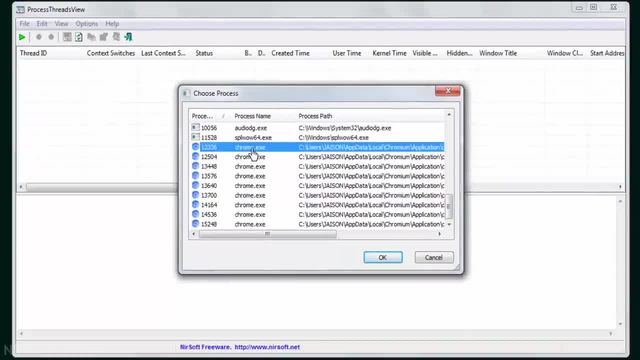 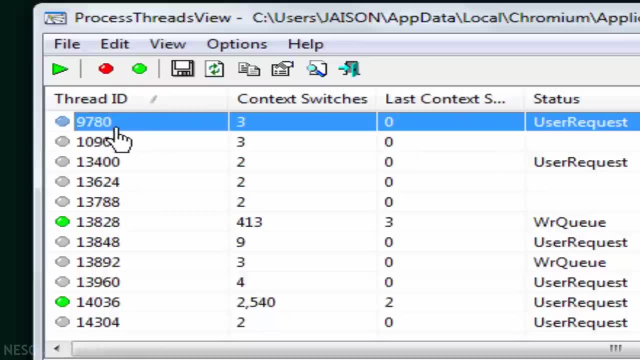 the system. Now, if I want to see the thread associated with it, I will just click on it and it will show me the thread associated with it. So I can see the thread associated with it, And here the details about the thread is populated. So there are this many number of 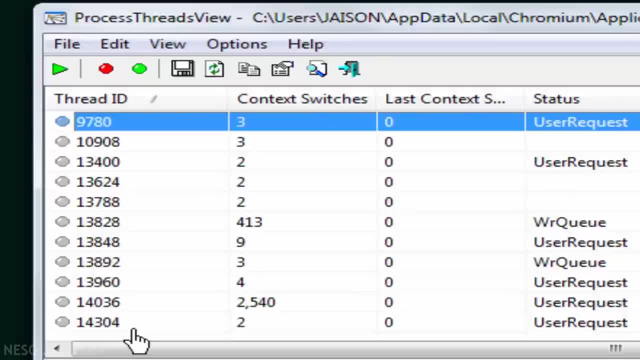 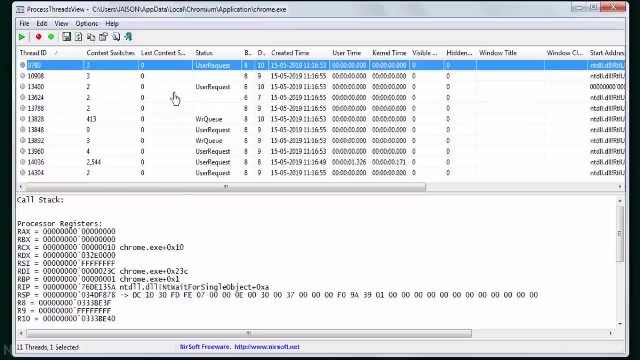 threads associated with that single chromeexe process that was running. So, as I told you, the thread comprises of a thread id. So these are the ids of the thread, which identifies those threads uniquely, And then these are the context switches and the last context switches that happen. So we 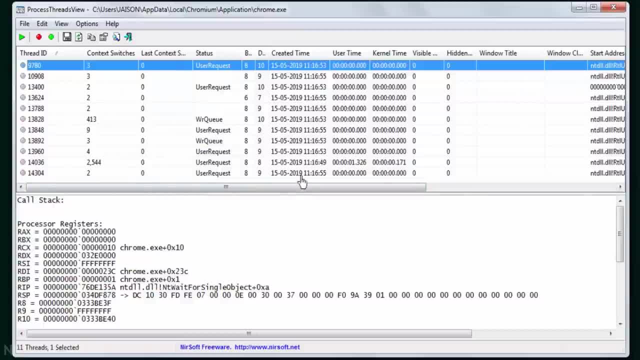 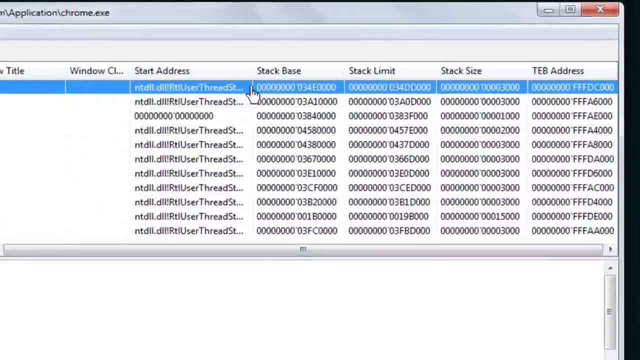 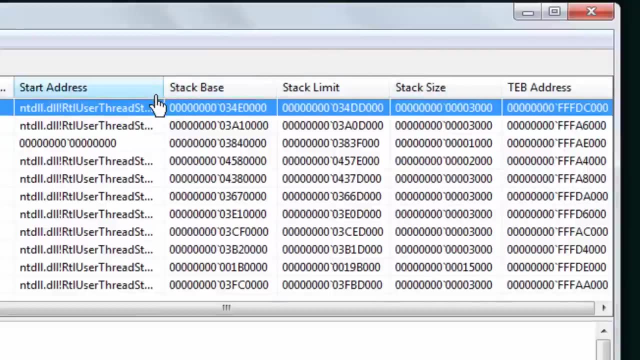 have discussed about context switches in one of the previous lectures, And here there are so many things about the thread that we have selected. Now, if we come here, we can see that there is the address of the thread And here we can see the details of the stack associated with that process. 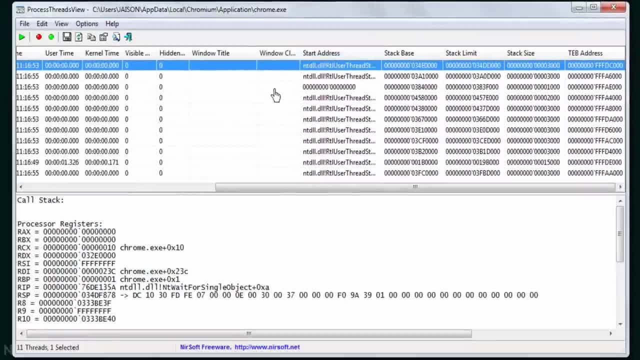 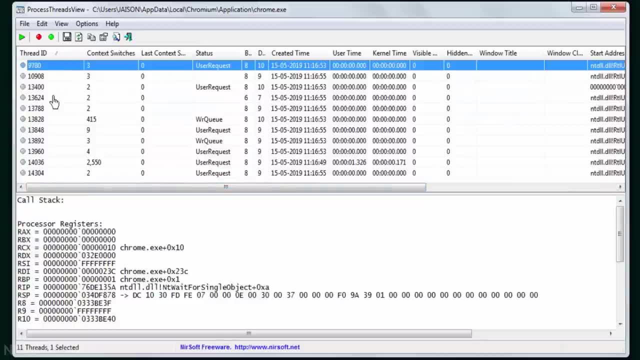 So I told you that threads also contain a stack. So in this way we can see what are the processes running in our system And we can also see the threads associated with those processes. So we clearly see that in this system it is following a multi-threaded approach. So when I clicked that, 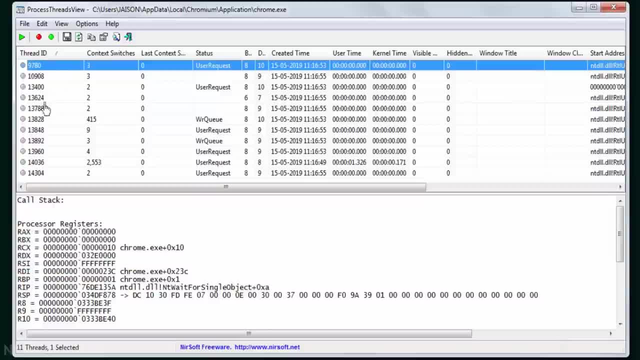 single process of that chromeexe, we see that this many number of threads are running inside that process. So each of these threads may be used for performing a different task. So in that way the browser can do more than one task at a time. So let's say, for example, one of the processes of 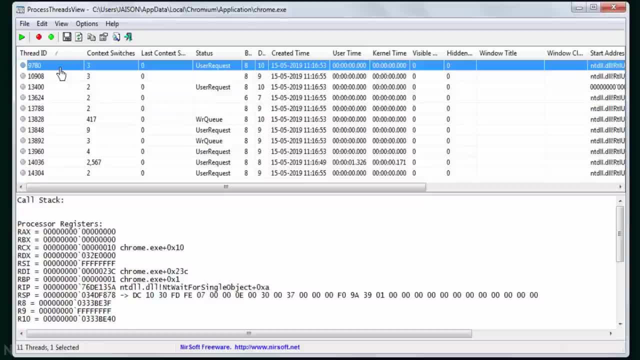 this browser, chromeexe, is used for displaying the web page on the browser window, And let's say that another thread is used for downloading something from the internet. So we know that when we are downloading something, we can also view the page at the same time. So these two things are happening. 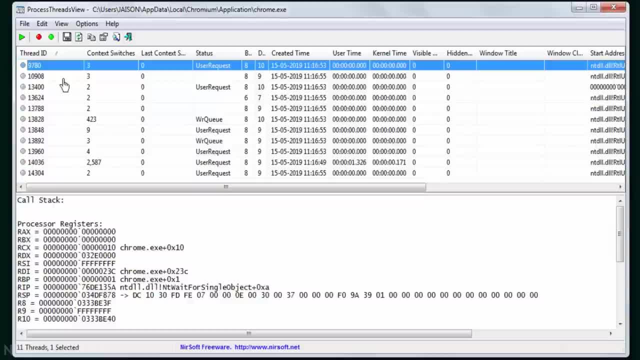 simultaneously. That is possible because we are having multiple threads: One thread is taking care of displaying and the other thread is taking care of downloading. So if we were having only a single threaded process, then while the downloading was happening, the page could not be displayed Or 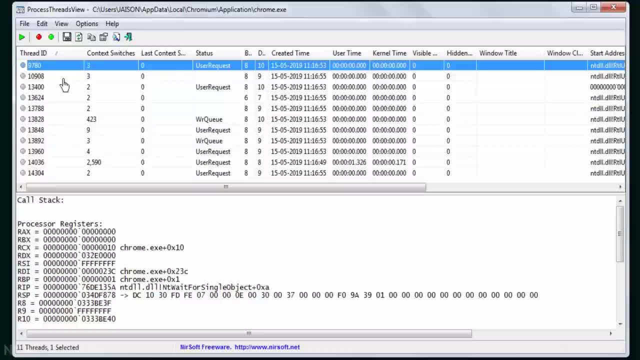 while the page is being displayed, the download will not happen. So that is just a simple example that I want to take in order to make us understand the usage of multi-threaded processes. So let's go ahead and see what are the benefits of multi-threaded processes. So different threads perform different tasks, and 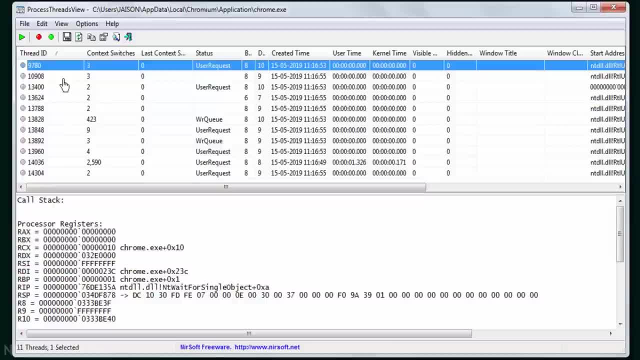 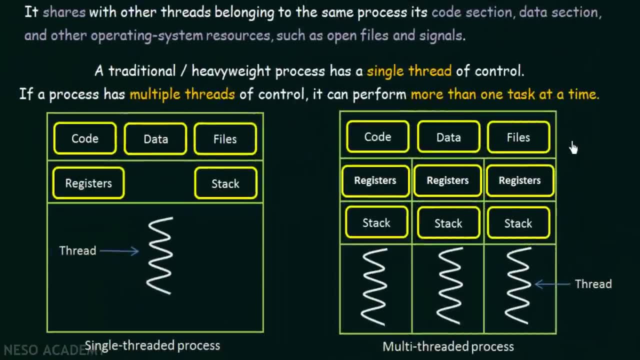 hence multiple tasks can be performed at the same time, Hence improving our efficiency and speed of computation. So we have seen a visual example of how multi-threaded processes are there in our system. Now let us see what are the benefits of having multi-threaded processes. So, from the 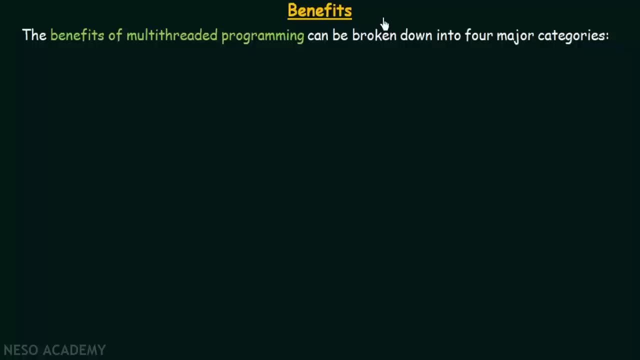 example that I have taken. you must have already understood the benefits of using multi-threaded processes, But let us understand these benefits in more detail. So the benefits of multi-threaded programming can be broken down into four. The first benefit of multi-threaded programming is that the 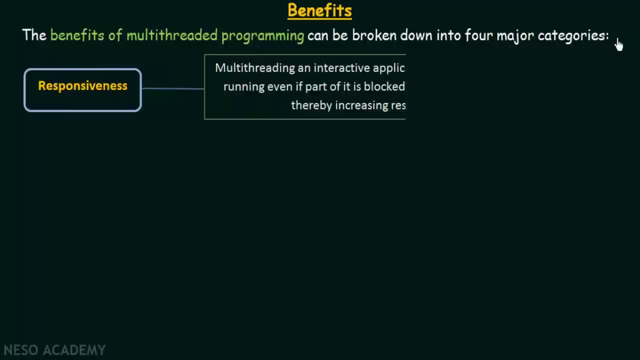 four major categories, So let's see what they are one by one. So the first benefit is responsiveness. Multi-threading- an interactive application, may allow a program to continue running even if part of it is blocked or is performing a lengthy operation, Thereby increasing responsiveness. 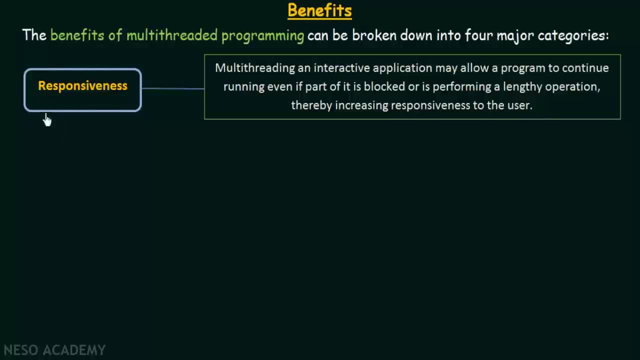 to the user. So we are having a better responsiveness if we have multi-threading. So I can explain this using the same example that I took about the web browser, Since we said that we are having different threads, one for displaying the web page and another one. 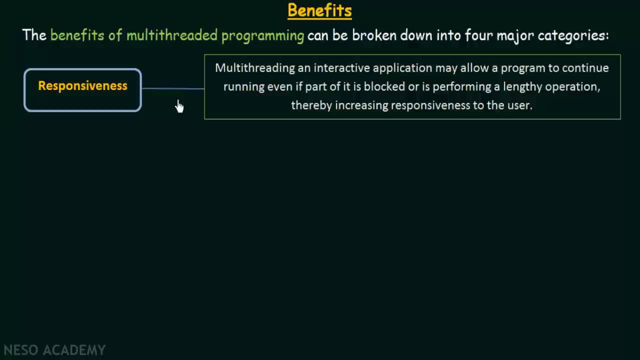 for downloading and, let's say that, another one for the user to interact with the web page. So if only one thread was there, then until and unless one of the tasks completes, the other task cannot be done. So the user have to wait for one of the tasks to be complete in order to go to the next. 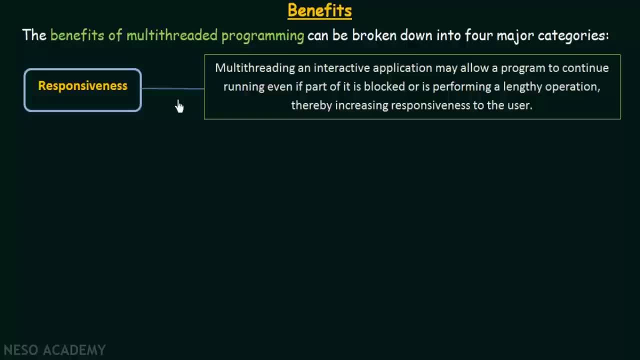 task. But in case of multi-threading, since different threads are simultaneously performing different tasks, the responsiveness to the web page will be increased. So we are having a better responsiveness to the user increases. So that is the first benefit of multi-threaded programming. 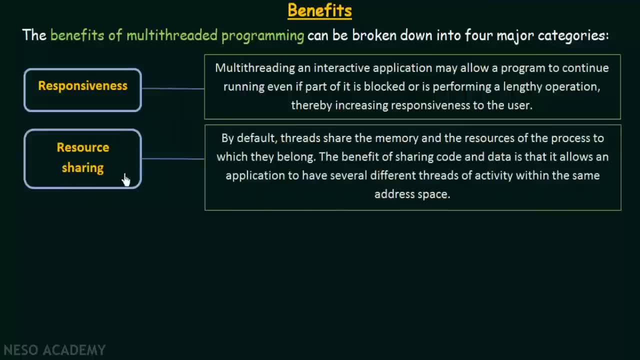 So let us see what is the next benefit. So the next benefit is resource sharing. So, by default, threads share the memory and the resources of the process to which they belong. The benefits of sharing code and data is that it allows an application to have several different threads. 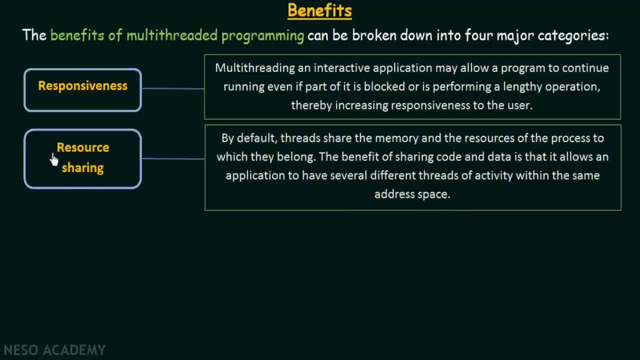 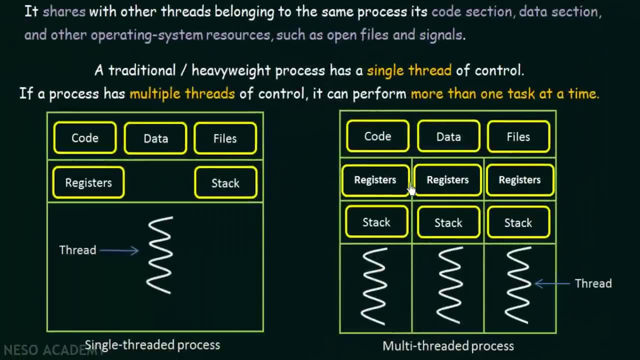 of activity within the same address space. So the next benefit is resource sharing. So when we saw that these multiple threads, they are sharing the resources of the same process, So the code, data and files are shared between these three threads, So we said that it shares with other threads. 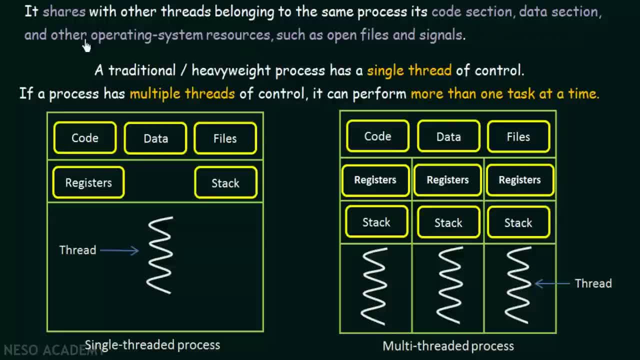 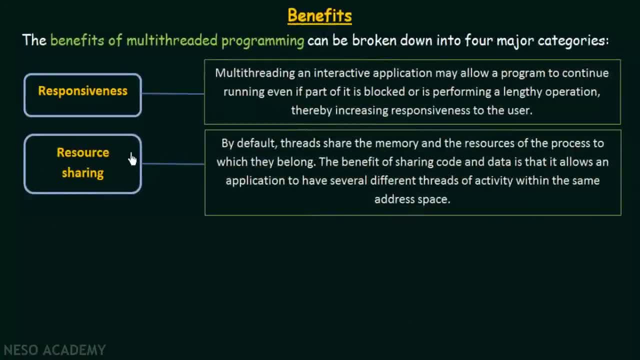 belonging to the same process: its code section, data section and other operating system resources, such as open files and signals. So we see that resource sharing is happening in multi-threaded programming. So the benefit of sharing code and data is that it will allow application. 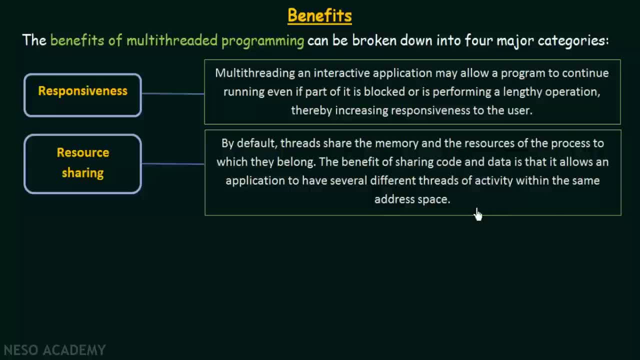 to have several different threads of activity within the same address space. So we can have several different threads in the same address space of the same process. So by resource sharing we are making our system more efficient because it does not need to have separate or dedicated. 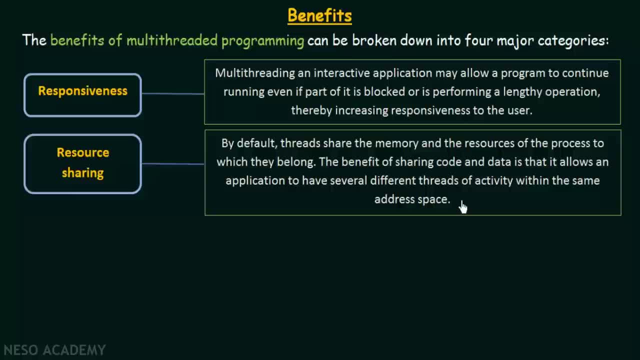 resources for each and every threads, So sharing resource is another benefit of multi-threaded programming. So, coming to the next benefit, we have economy, So allocating memory and resources for process creation and processing is another benefit. Is there any other benefit that we could? 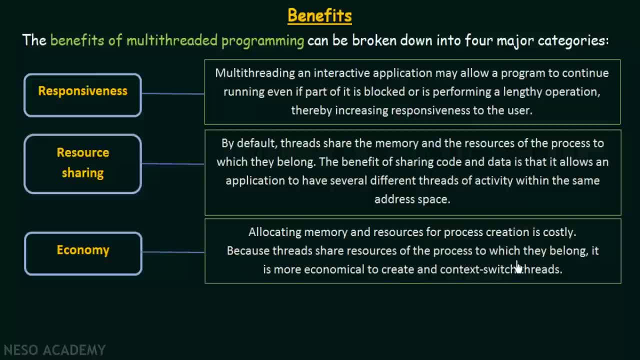 is costly because threads share resource of the process to which they belong. It is more economical to create and context switch threads. So we already saw that there is resource sharing happening in case of multi-threading. So if there was no multi-threading then we will need to have 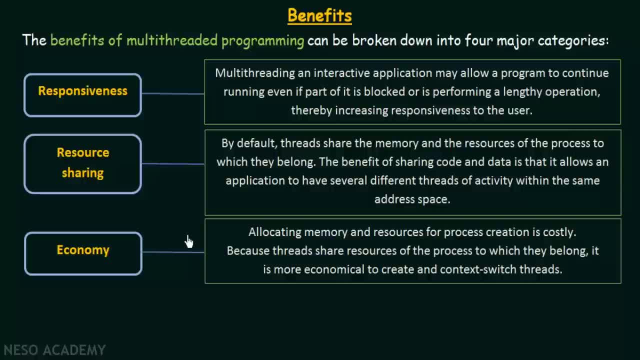 a separate process for each and every task that has to be performed, and allocating memory and resources for the processes is costly, because each process will need to have its dedicated resources and memory, which it may not be able to share with other processes. But in threads as they. 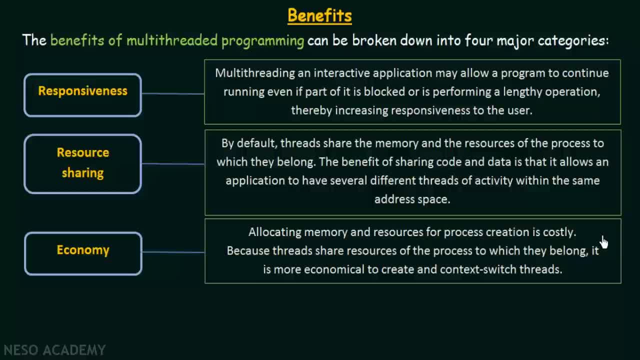 are able to share the resource of the processes to which they belong. it is more economical to create and switch between threads because we don't need to have those dedicated resources. they are able to share and hence it is economic. So this economy, it comes from this resource. 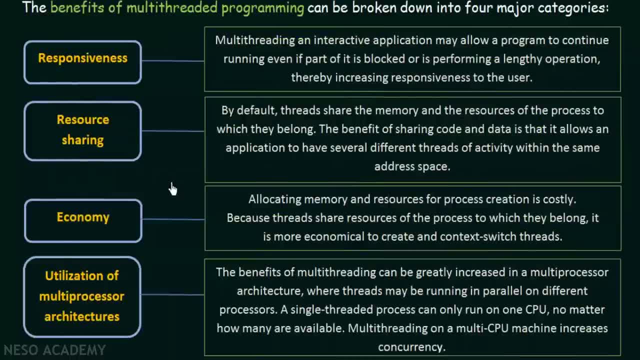 sharing. Now, moving on, the next and the last benefit that we have is utilization of multi-processor architectures. The benefit of multi-threading can be greatly increased in a multi-processor architecture, where threads may be running in parallel on different processors. A single threaded process can only run on one CPU, no matter how many are available. Multi-threading- 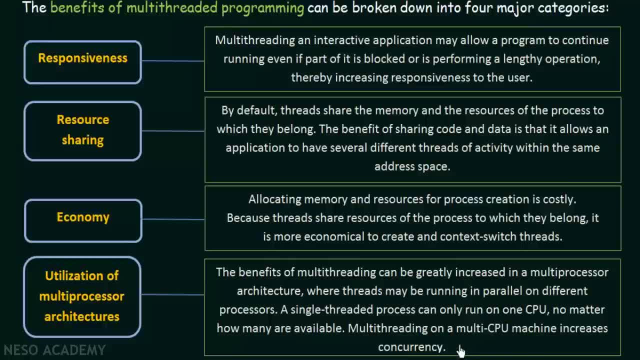 on a multi CPU machine increases concurrency. So the next benefit we have is utilizing of multi processor architecture. So we have already studied about multi-processor architecture in this lecture series of operating system. So multi processor architecture means there are several number of processors in our system. But if we are not having a multi-threaded 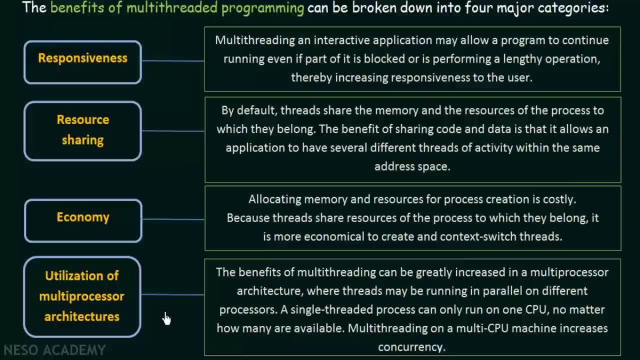 approach and instead having a single threaded process, then what will happen is that if we are having one process, that one process can run on only one processor or on one CPU. So you may have different CPU. So let's say you want to run on one processor, So let's say you have a single. 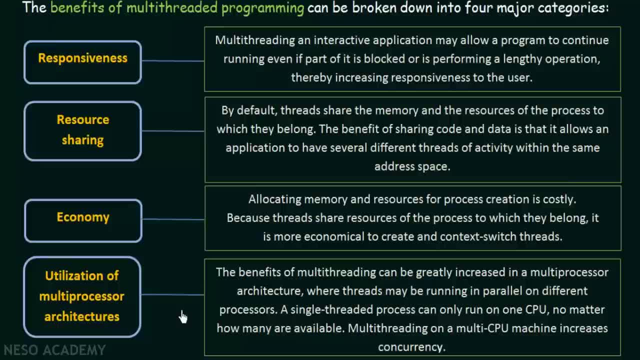 for example, that we are having four processors in your system. But even though you are having four processors, since your process is a single threaded process, that single process can run only on one of the processor. So no matter how many number of processors you may have, 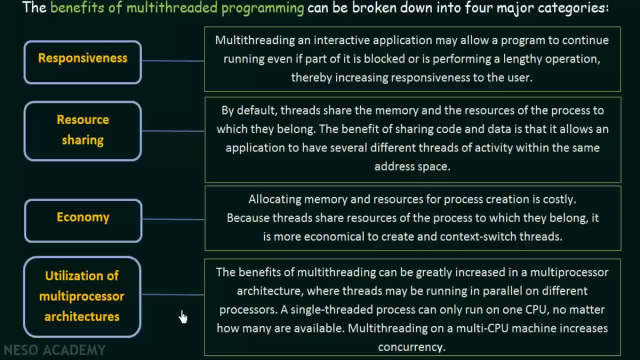 having a single threaded process will run in only one of the processor. But if we are having a multi-threaded approach, then what will happen is that we know that in a multi-thread approach, each process has a different number of threads associated with it, So each of these threads 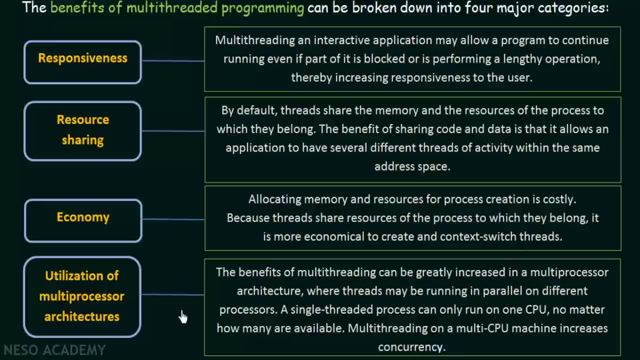 can run on these multiple processors. Let's say that there are four threads associated with a single process and then there are four processors in your system, So each of those threads can run on one of the processors. So thread 1 may run in processor 1, thread 2 may run in processor 2. 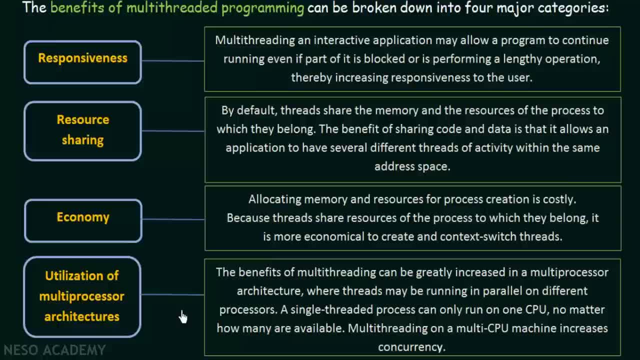 and so on. So in this way, we see that the tasks are executed concurrently at the same time, and hence the process will be completed quicker and it is more efficient. That is what we mean by utilization of multi-processor architecture. So if we don't have a multi-threaded approach, 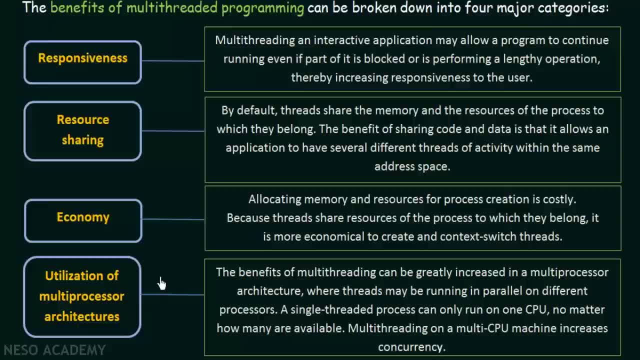 even though we have multi-processors, it is not very useful because we are not able to make use of the multi-processor architecture. But in case of multi-threading, we are able to make use of multi-processor architecture, hence improving our.